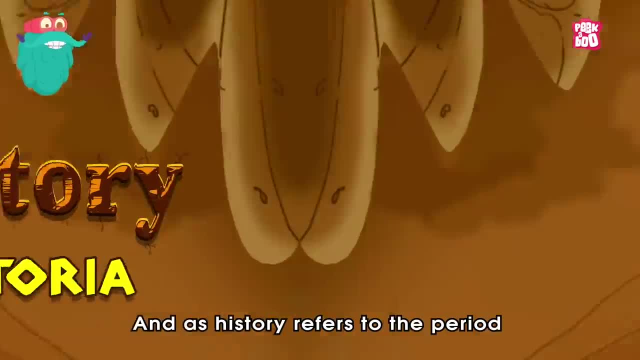 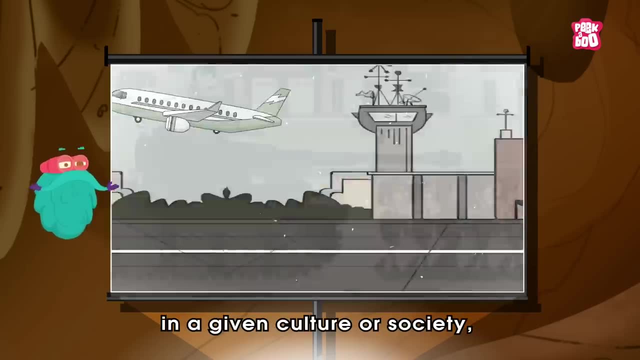 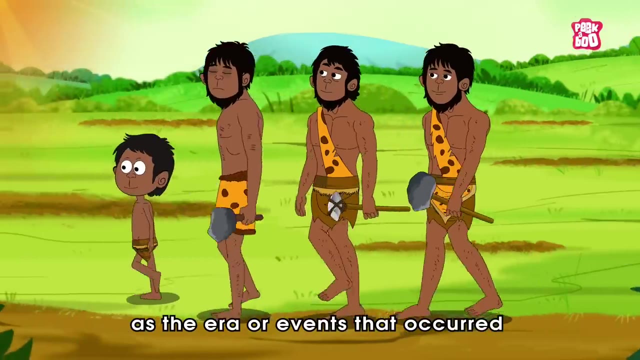 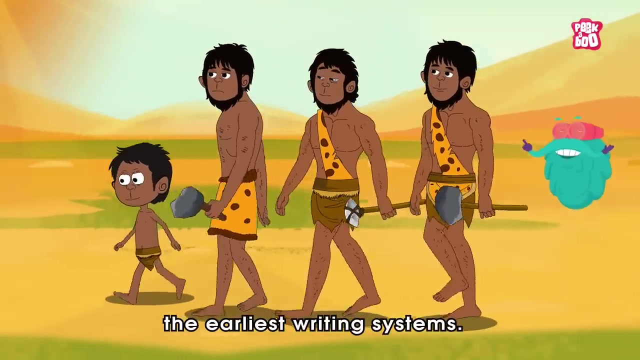 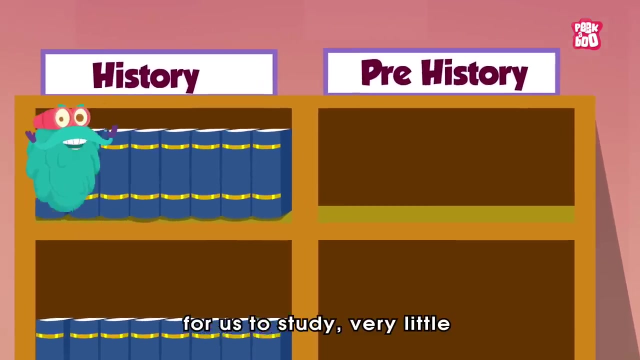 translates to history And, as history refers to the period after the invention of written records in a given culture or society, It means we can define prehistory as the era or events that occurred before the development of the earliest writing systems. Unfortunately, due to no written records for us to study, very little is known about prehistoric. 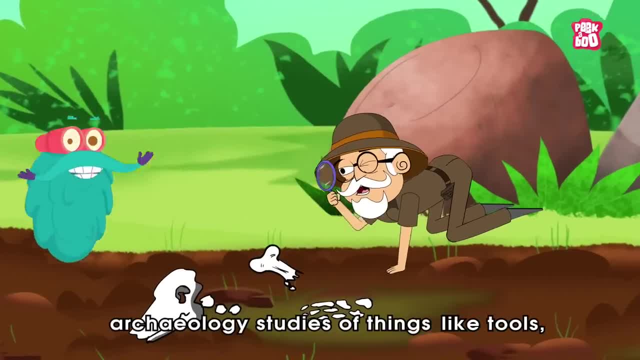 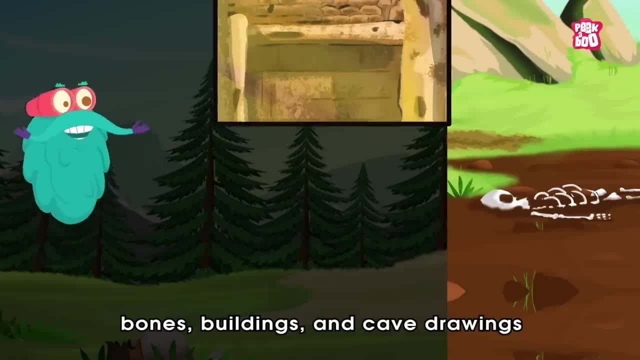 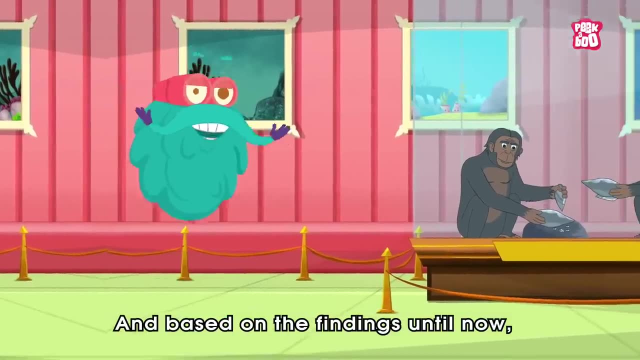 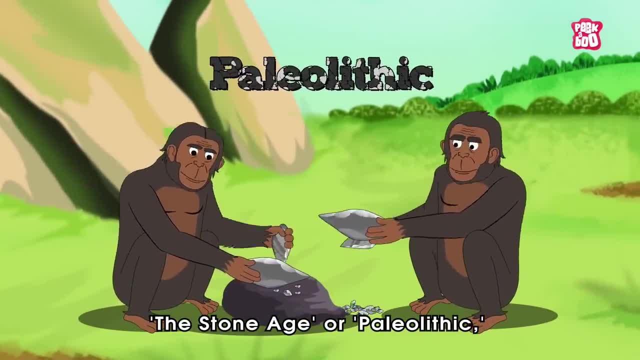 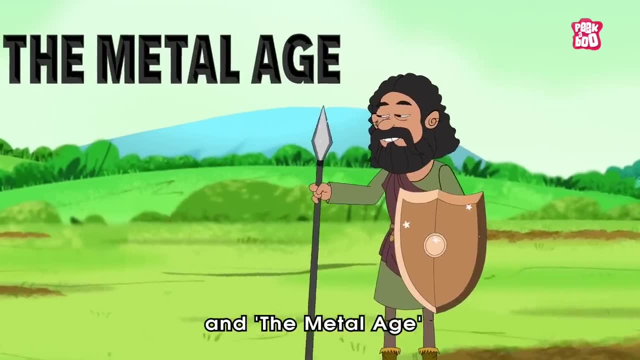 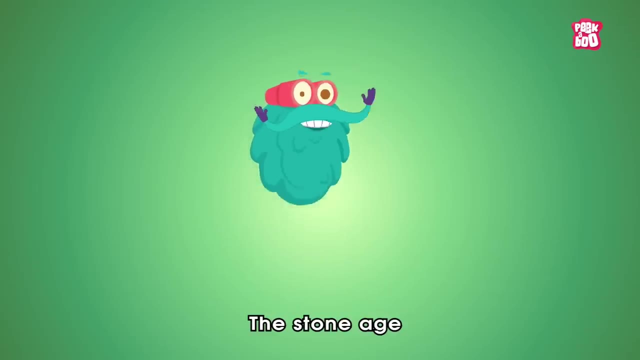 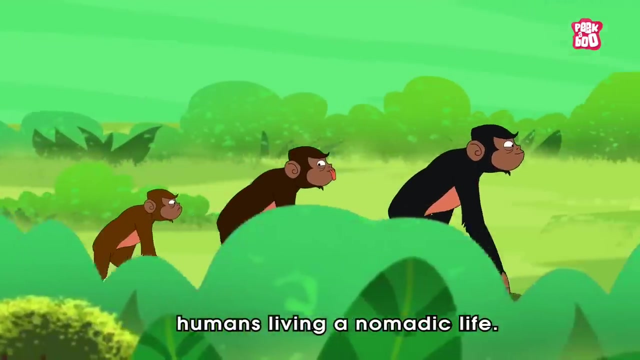 Namely the Stone Age or Paleolithic, the Agricultural Revolution, or the Neolithic and the Metal Age, which consisted of the Bronze and Iron Age. The Stone Age began nearly 2.6 million years ago with the rise of the first humans living a nomadic life. 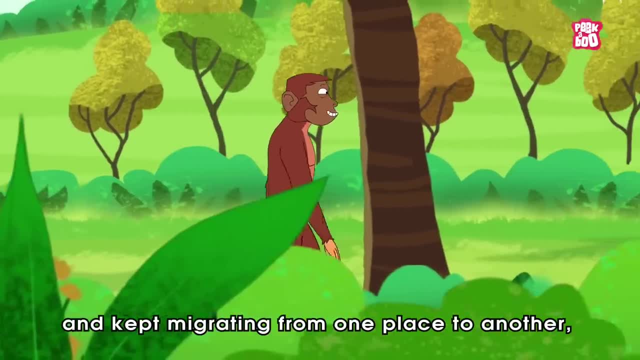 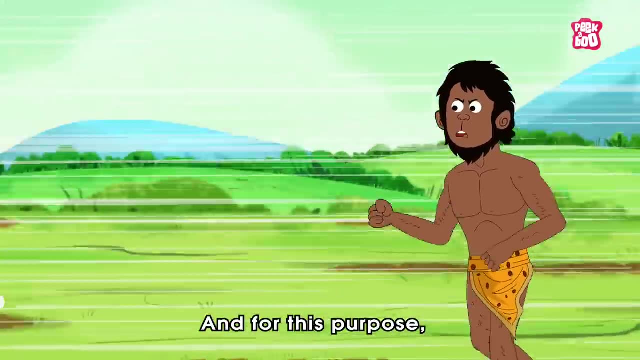 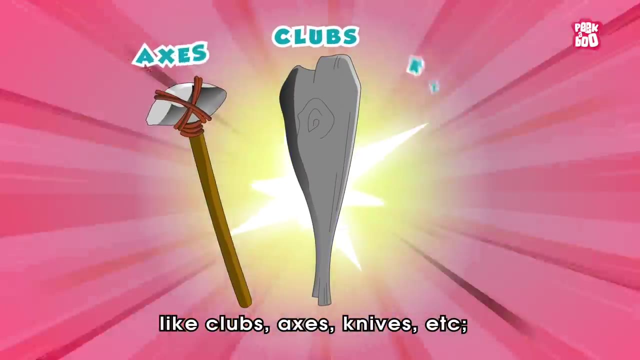 This means that they never settled in one place and kept migrating from one place to another, especially for hunting, And for this purpose they started using stones to make tools like clubs, axes, knives, etc. And for the same reason we call it a Stone Age. 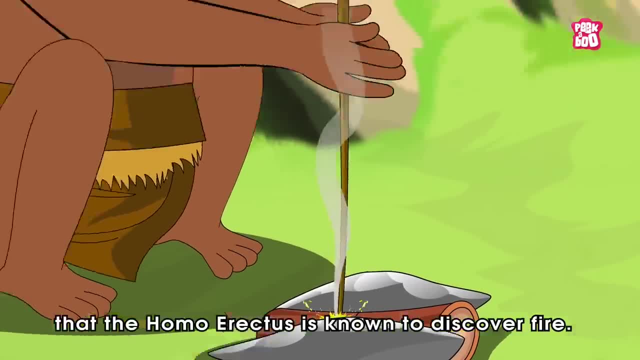 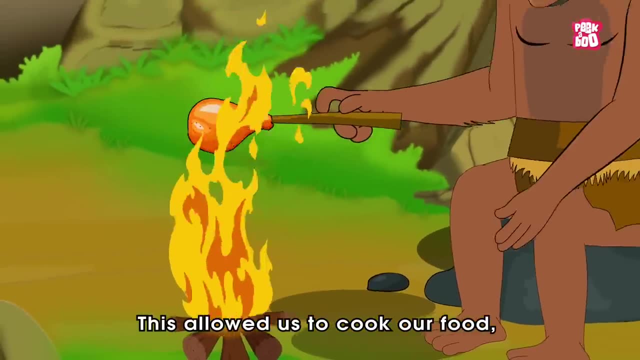 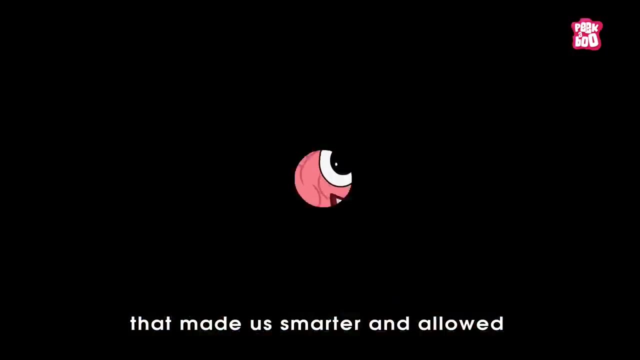 And it is in the Stone Age that the Homo erectus is known to discover fire. This allowed us to cook up food, which may be the main factor behind the development of our brains. that made us smarter and allowed us to enter the next stage. 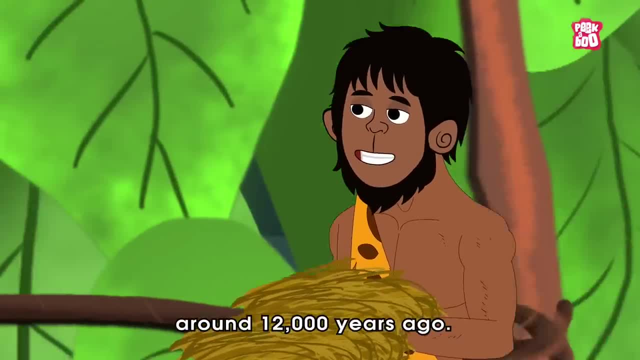 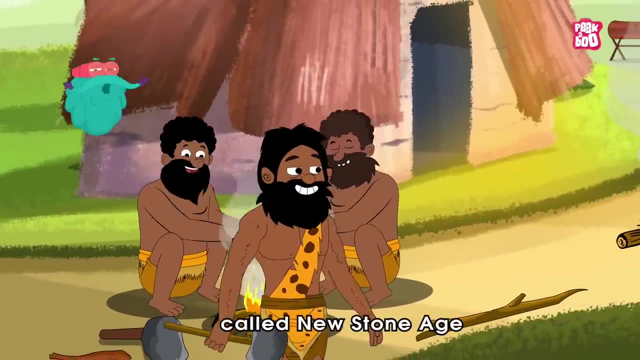 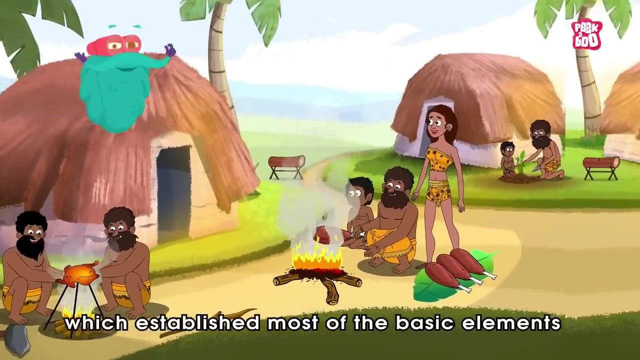 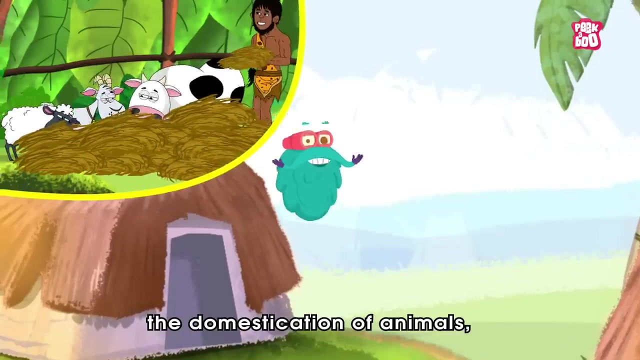 the Neolithic period, which started around 12,000 years ago. The Neolithic period, also called New Stone Age, was an era of technological and social developments which established most of the basic elements of historical cultures, such as the domestication of animals. 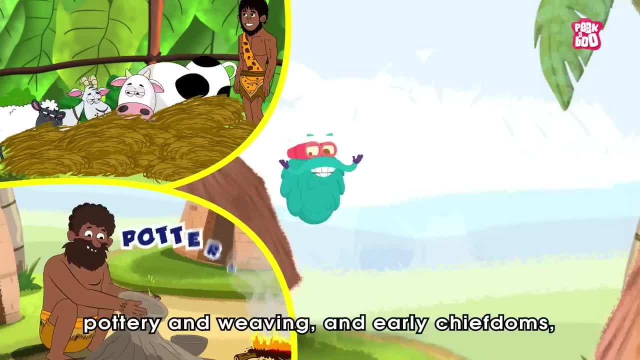 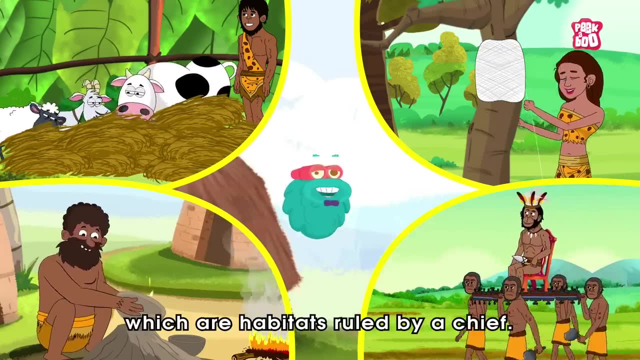 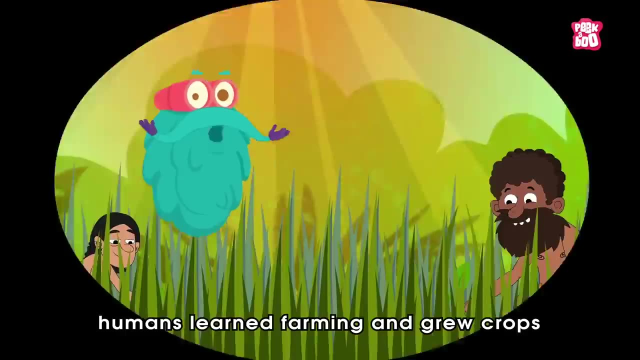 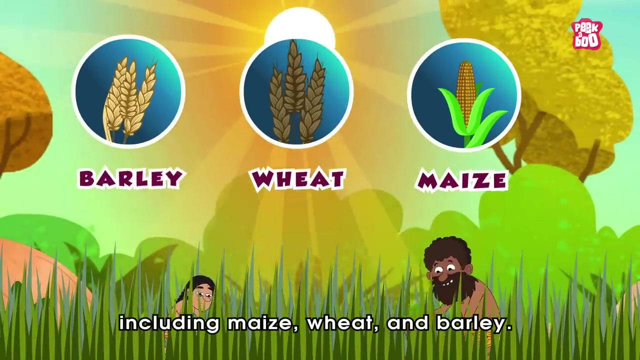 the appearance of crafts such as pottery and weaving, and early chiefdoms, which are habitats ruled by a chief. But, more importantly, during the Neolithic period, humans learnt farming and grew crops, including maize, wheat and barley. This led to the construction of small villages where Homo sapiens 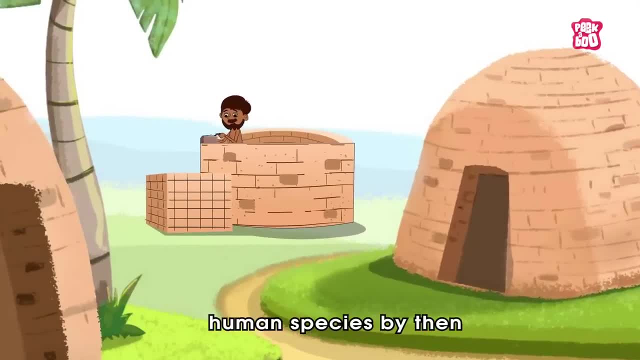 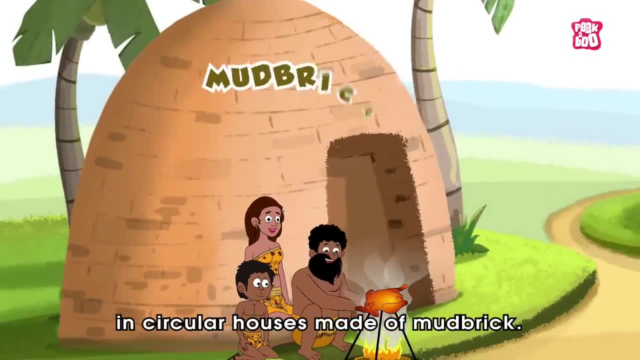 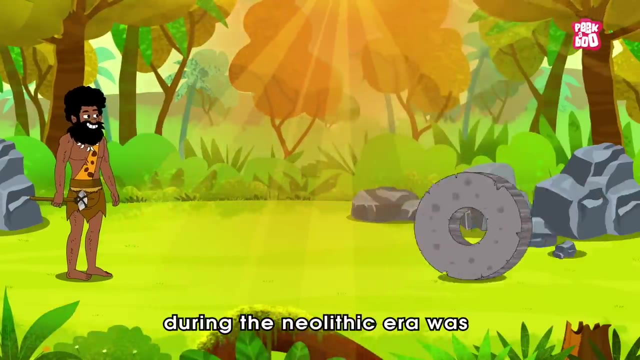 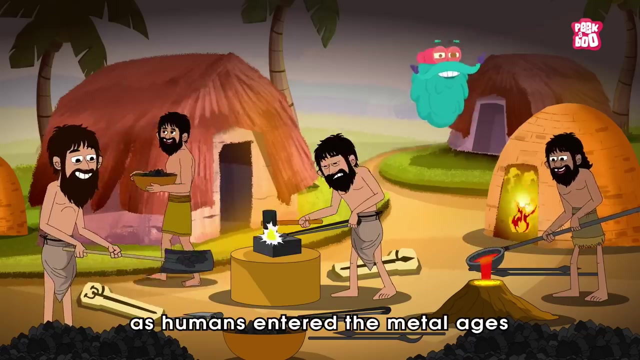 probably the only left. human species by then began to settle permanently in circular houses made of mud brick. Another important innovation that happened during the Neolithic era was the invention of the wheel. This drove the development further as humans entered the Metal Ages that started approximately 6,000 years ago. 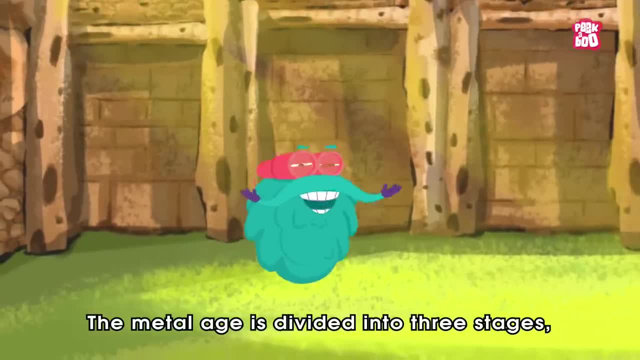 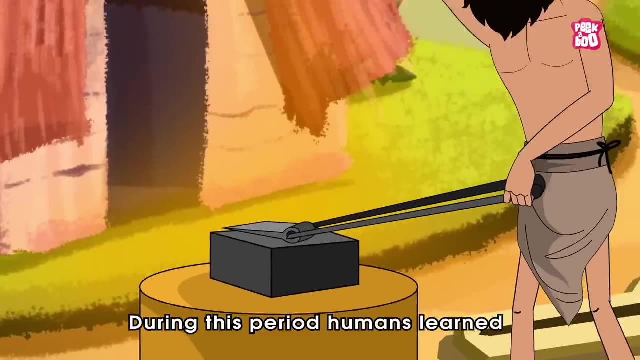 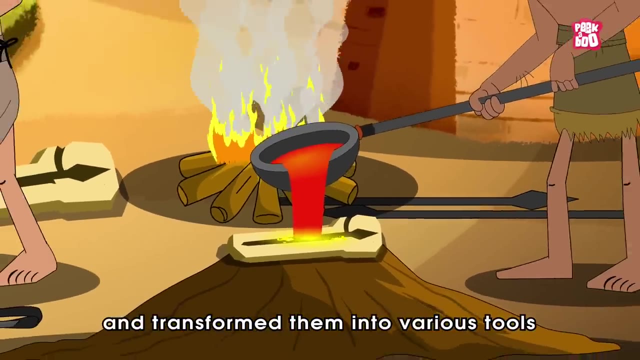 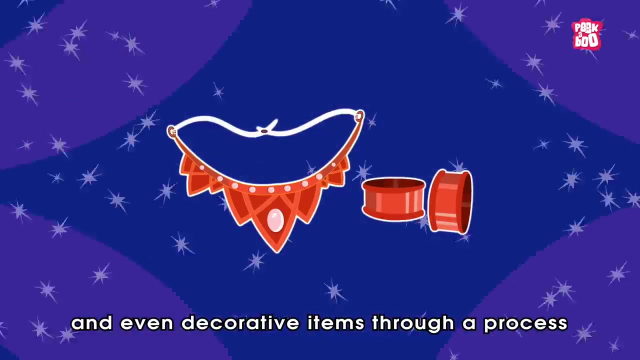 The Metal Age is divided into three stages: the Copper Age, the Bronze Age and the Iron Age. During this period, humans learnt to heat the metals at extreme temperatures and transform them into various tools like weapons, vessels and even decorative items through a process called metallurgy. 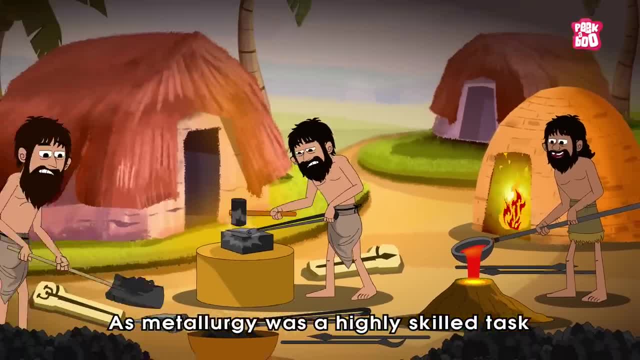 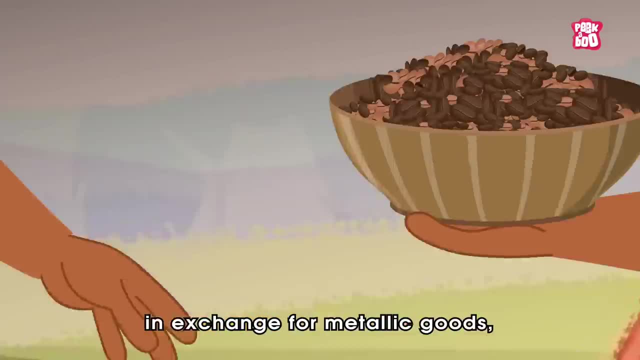 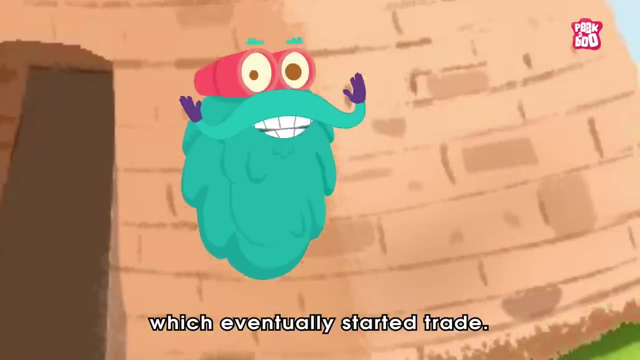 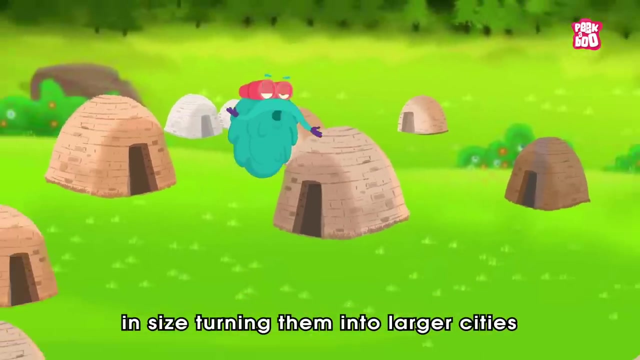 As metallurgy was a highly skilled task only known to a few other people, began to swap agricultural products in exchange for metallic goods, giving rise to the barter system which eventually started trade. Trading then helped small villages to grow in size, turning them into larger cities.